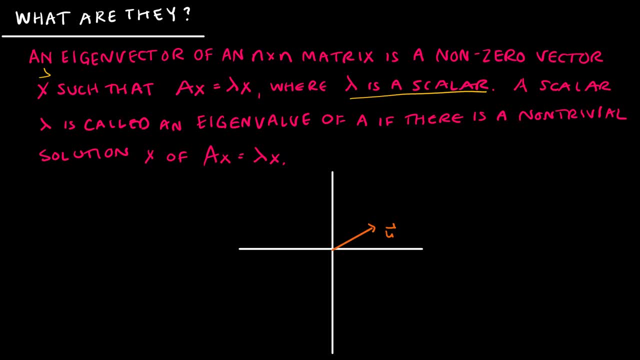 and lambda is just a scalar. In addition, the scalar itself is called the eigenvalue if there is a non-trivial solution, x for that equation. ax equals lambda x. So before we look at you know, making sense of all of this, let's make sure we understand graphically what's happening. 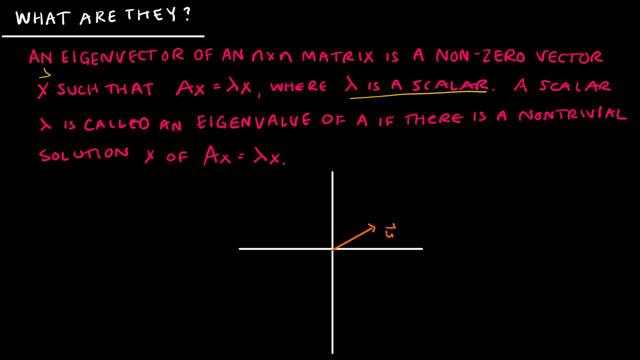 So if I have some vector u- or I guess I could have called it vector x- essentially I'm going to have a vector x that is non-zero, such that ax equals lambda, x for some lambda. essentially, what we're saying is that lambda is going to be some scalar, which might make you. 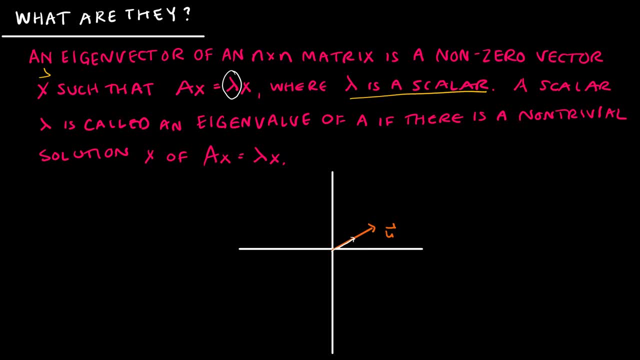 compress a little bit or stretch or possibly go in the opposite direction, And so, essentially, lambda is going to create our resulting vector somewhere along that line. So now let's take a look at mathematically: what does this do for us? The first thing we can do is to determine if x 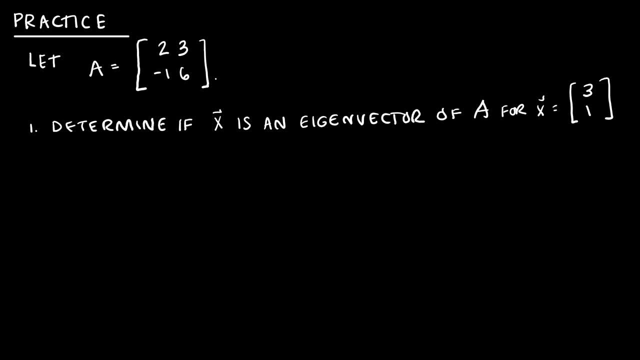 is an eigenvector of a and they've given us an x vector. So I have a: is 2, 3, negative, 1, 6.. And my question is: is x, 3, 1, an eigenvector of a? So all we have to do here, if you'll recall, we said that ax. 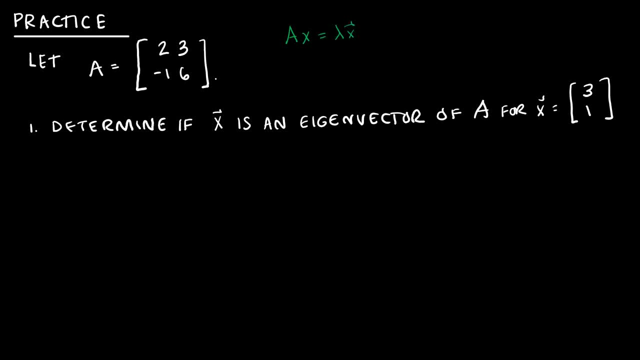 had to be equal to lambda x, And so I'm going to take ax and see what happens. In this case, that's 2,, 3, negative 1, 6, and then 3, 1.. And we all know how to multiply matrices. 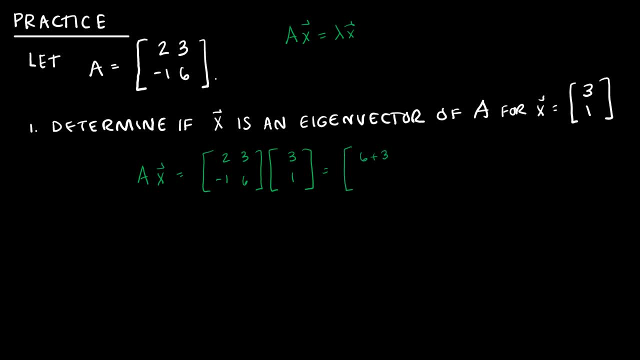 So I'm going to get 6 plus 3, and negative 3 plus 6, and that gives me 9, 3.. So ax is 9, 3.. The question is: is that equal to some scalar times x? Well, I can see that 9, 3. 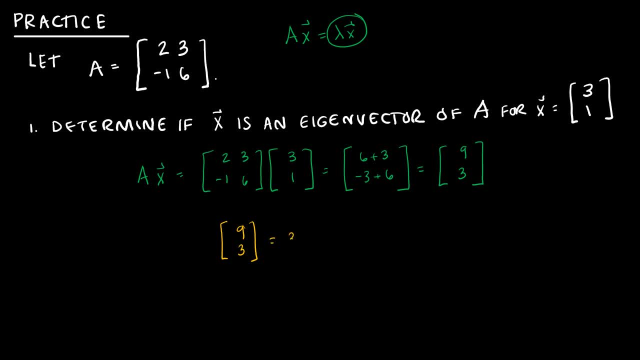 can be written as 3 times 3, 1.. And 3, 1 is actually just x from the question. So is x an eigenvector of a. And then I'm going to take x, 3, 1, 6, and then 3, 1.. And I'm going to take x 3,. 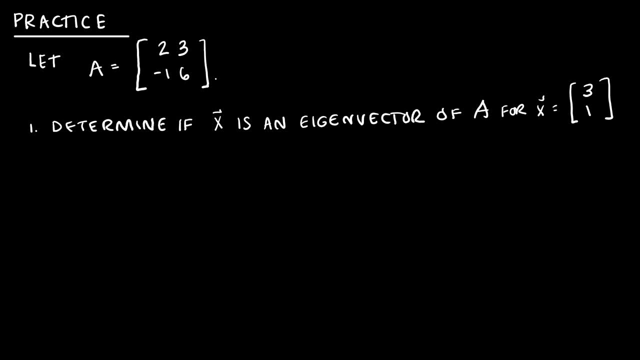 is an eigenvector of a and they've given us an x vector. So I have a is 2, 3, negative 1, 6, and my question is: is x, 3, 1, an eigenvector of a? So all we have to do here, if you'll recall. 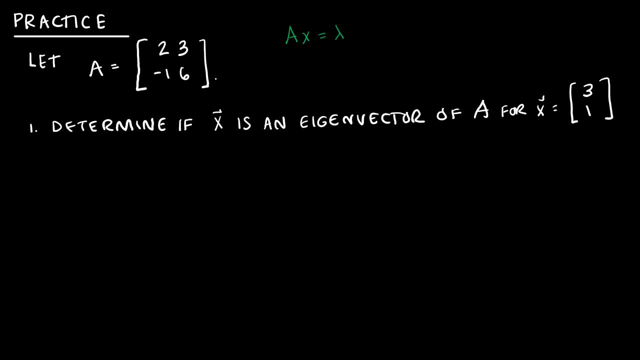 we said that ax had to be equal to lambda x for some lambda x, and we said that x had to be equal to lambda x for some lambda x, And so I'm going to take ax and see what happens. In this case, that's 2, 3, negative 1, 6, and then 3, 1, and we all know how to. 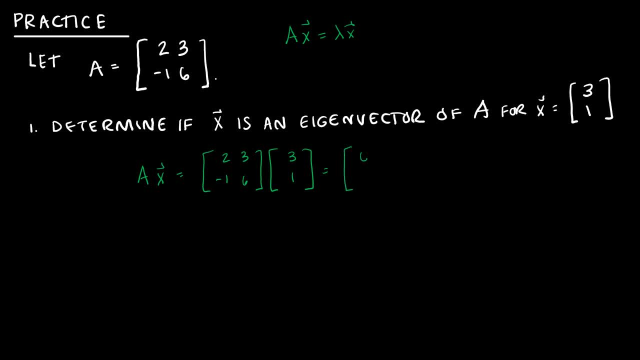 multiply matrices. So I'm going to get 6 plus 3, and negative 3 plus 6, and that gives me 9, 3.. So ax is 9, 3.. The question is, is that equal to some scalar times x? Well, I can see that 9, 3 can be written. 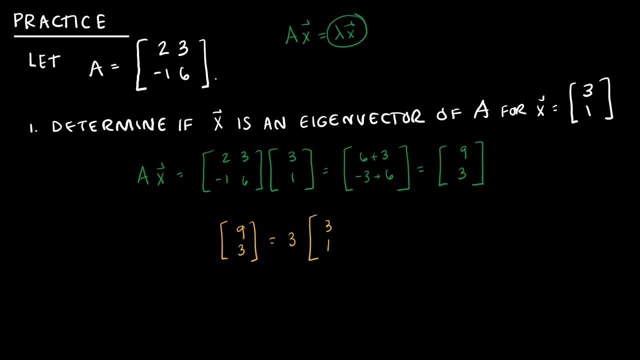 as 3 times 3, 1, and 3, 1 is actually just x from the question. So is x an eigenvector of a? Absolutely, because 3, is my eigenvalue and I can take 3 times x and that is equal to ax. So it really just fits the definition. 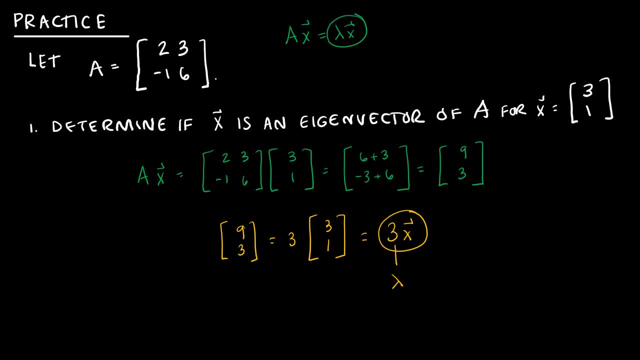 So that's how you're going to determine if some vector is an eigenvector is: you're just going to multiply a times x and see if it's equivalent to some lambda times x. Let's look at another question, and this one again is using my same matrix, a. 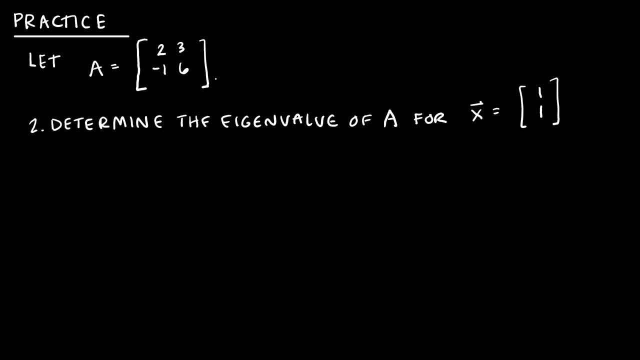 but I'm asking a different question. So I'm going to take a matrix a and I'm going to take a matrix a question. I'm asking to determine the eigenvalue of a for x, which in this case is 1, 1.. So in the 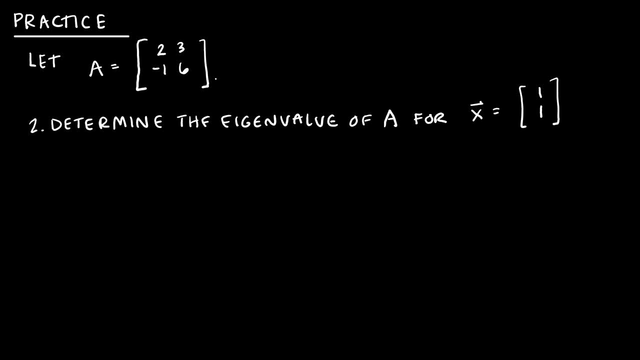 last question I was asked to determine if a vector was an eigenvector. Now I'm asking to find the eigenvalue, if one exists. So it could be that I ask you to find the eigenvalue and it doesn't exist, But in this case obviously I'm not going to do that. But the good news is we're. 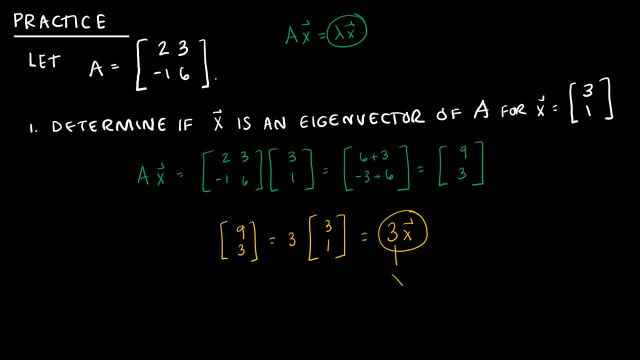 absolutely, because 3 is my eigenvalue And I can take 3 times x and that is equal to ax, So it really just fits the definition. So that's how you're going to determine if some vector is an eigenvector is: you're just going to multiply a times x and see if it's equivalent to some lambda. 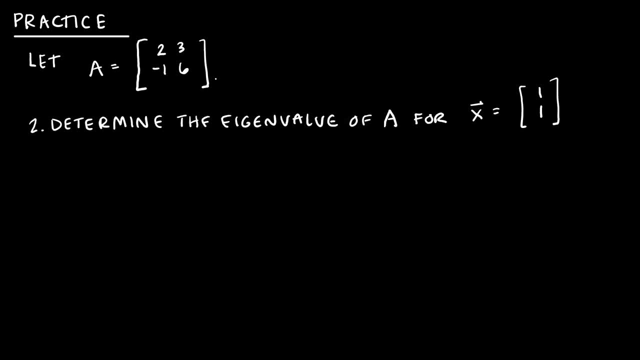 times x. Let's look at another question, And this one again is using my eigenvector, my same matrix, A, But I'm asking a different question. I'm asking to determine the eigenvalue of A for x, which in this case is 1, 1.. So in the last question I was asked to determine 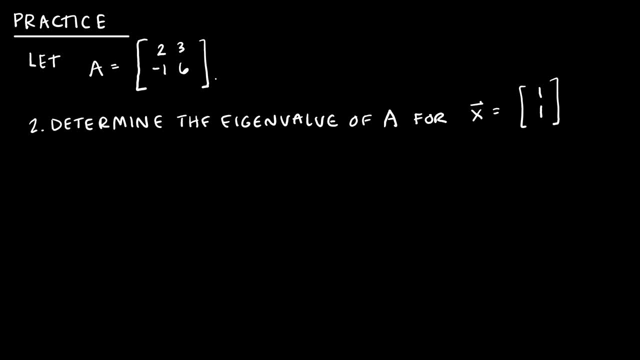 if a vector was an eigenvector. Now I'm asking to find the eigenvalue, if one exists. So it could be that I ask you to find the eigenvalue and it doesn't exist, But in this case obviously I'm not going to do that. But the good news is we're going to do this. 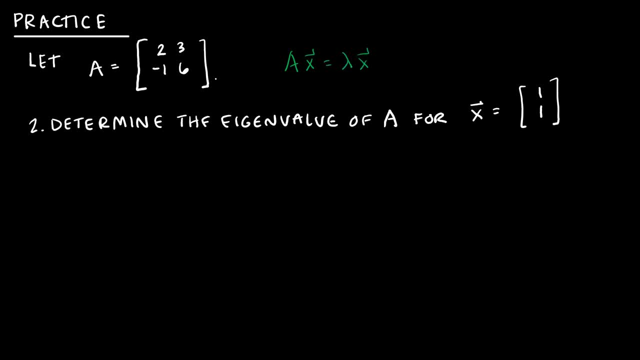 the same way that we did the last question, because I'm still saying that if an eigenvalue exists, then it's going to. you know, then A times x is going to be equal to lambda times x for some lambda, And, of course, the eigenvalue is just lambda. So all I'm going to do is exactly what. 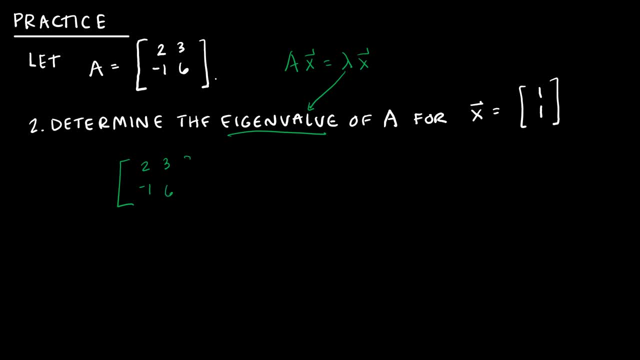 I did in the last question. I'm going to take A, I'm going to multiply it by x And that's going to give me, in this case, 2 plus 3 and negative 1. Plus 6.. And that gives me 5,, 5.. And, just like I did last time, I'm saying is 5, 5,. are we able? 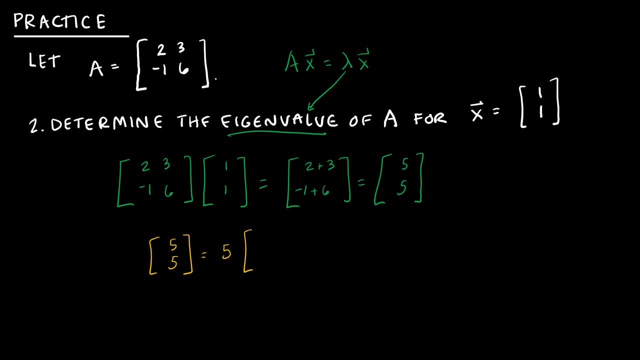 to write that as some scalar times vector x And of course this is 5 times 1, 1,, which is 5 times vector x, And therefore the eigenvalue lambda is 5.. So we could have easily been asked: is x an? 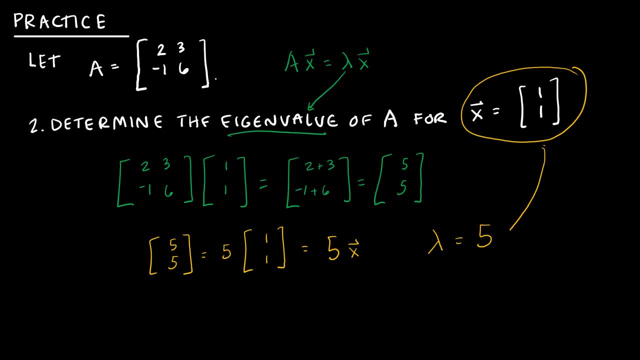 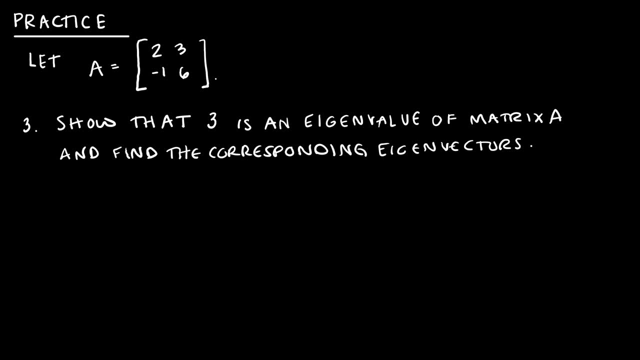 eigenvector And we would say yes, Or what is the eigenvalue? And the eigenvalue is 5.. Let's do a practice now. that's just a bit more difficult, And again we're still using that same equation that says A, x is going to equal lambda x if lambda is an eigenvalue, And of 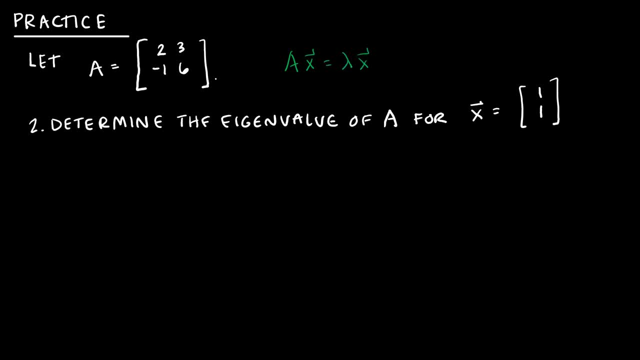 going to do this the same way that we did the last question, because I'm still saying that if an eigenvalue exists, then it's going to. you know, then a times x is going to be equal to lambda times x for some lambda And of course the eigenvalue is just lambda. So all I'm going 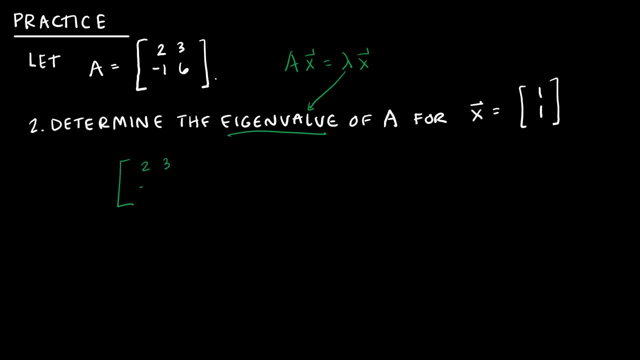 to do is exactly what I did in the last question. I'm going to take a, I'm going to multiply it by x And that's going to give me, in this case, 2 plus 3, and negative 1 plus 6.. And that gives me 5, 5.. And, just like I did last time, I'm saying is 5,. 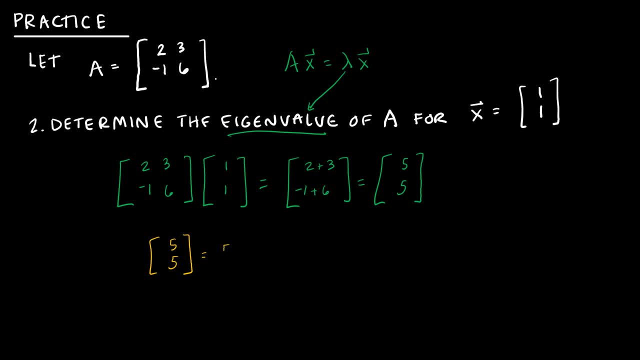 5, are we able to write that as some scalar times vector x? And of course this is 5 times 1, 1,, which is 5 times vector x, And therefore the eigenvalue lambda is 5.. So we could have easily. 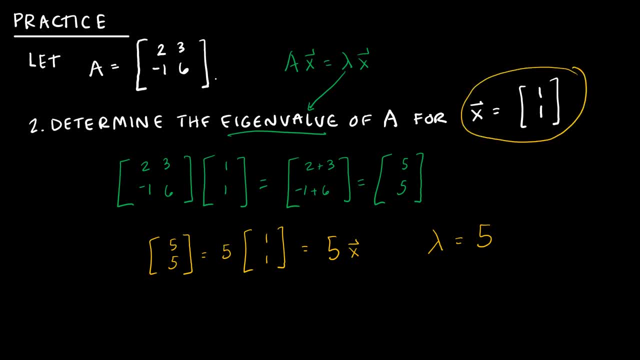 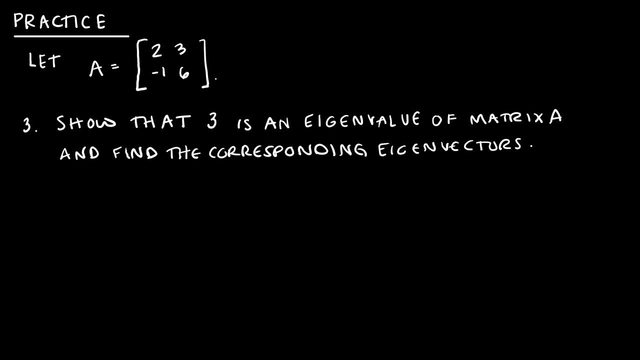 Let's do a practice now. that's just a bit more difficult. And again we're still using that same equation that says ax is going to equal lambda x if lambda is an eigenvalue. And of course that's what we're trying to do, is show that some value is an eigenvalue. 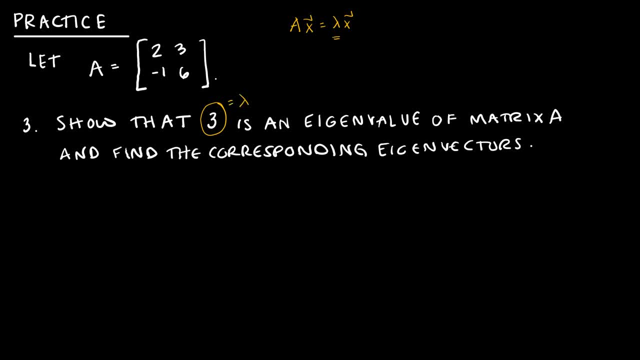 Now I've already done a practice like this in the opposite order. So our very first practice, practice one, actually used the same matrix A And instead it gave me a vector and said: is this an eigenvector? And then we had to solve to find an eigenvalue. This is the opposite of 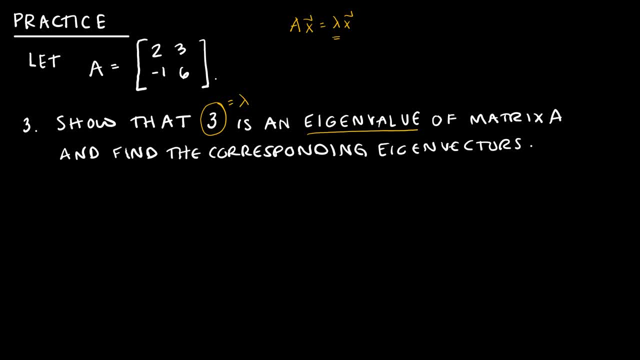 that. So here I'm giving you an eigenvalue And we already know in this case it's an eigenvalue because we did a practice like this. So we're going to solve to find an eigenvalue And we're going to solve to find an eigenvalue, And we're going to solve to find an eigenvalue, And we're 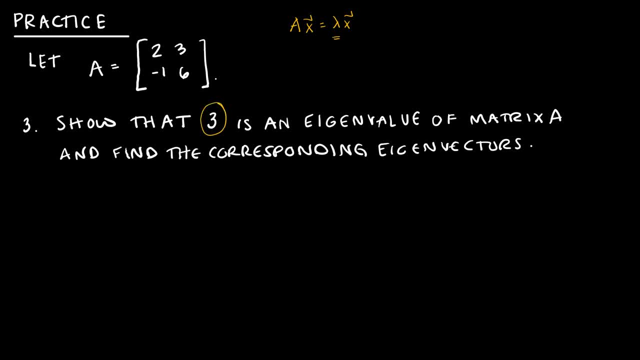 course that's what we're trying to do, is show that some value is an eigenvalue. Now, I've already done a practice like this in the opposite order. So our very first practice- practice 1, actually used the same matrix A And instead it gave me a vector and said: 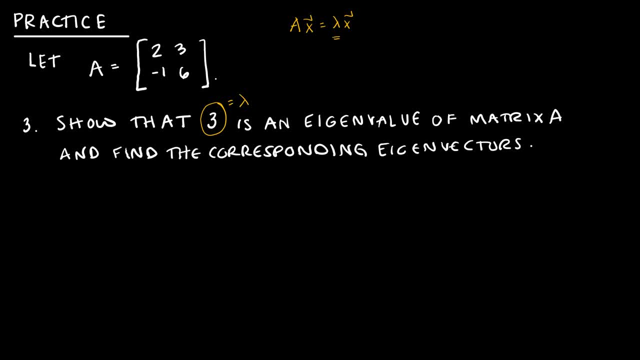 is this an eigenvector? And then we had to solve to find an eigenvalue. This is the opposite of that. So here I'm giving you an eigenvalue And we already know. in this case it's an eigenvalue because we did practice 1.. 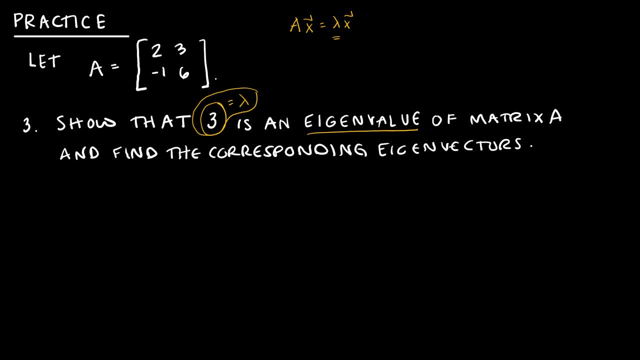 But typically you won't know that And you would have to show that it was true. You might be asking: how do we do that? Well, I'm glad you asked, We're still using this equation And we're going to say: well, if that's true, then A x minus lambda x must be equal to 0.. 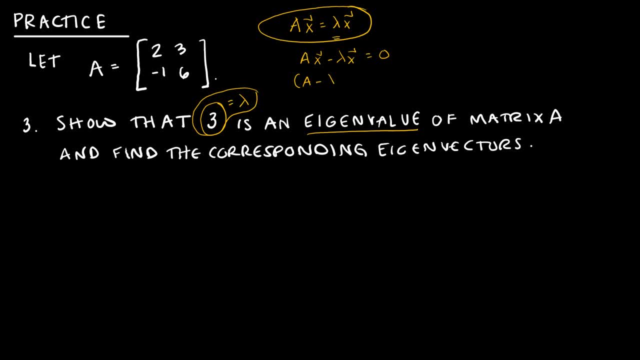 And then I could say: well, A minus lambda x is equal to 0.. But can I really take A, which is a matrix, and subtract lambda, which is a scalar? No, I can't. So what am I going to do? 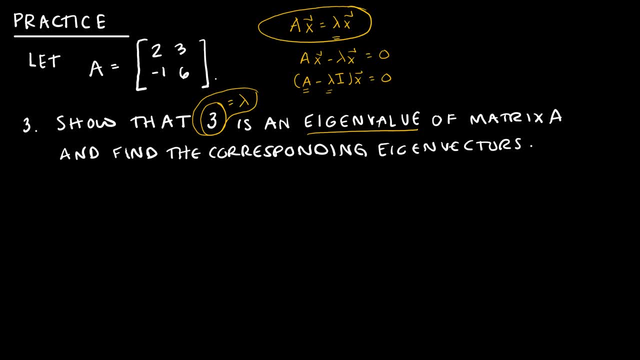 I'm going to take lambda times, the identity matrix. So for, obviously, a 2 by 2,. my identity matrix is 1, 0, 0, 1.. So here's how this is going to work. I'm going to take A which is 2, 3,. 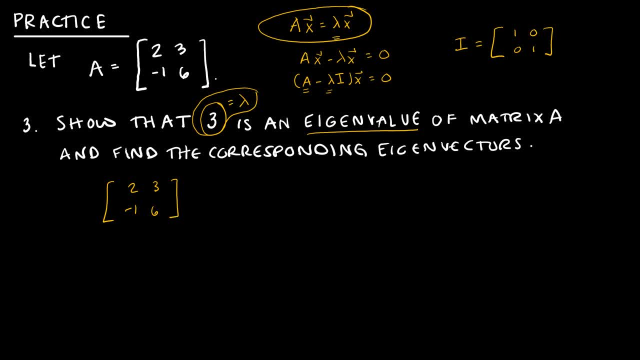 negative 1, 6.. And I'm going to subtract lambda, which is 3, times the identity matrix. So I'm going to take 3 times the identity matrix and get 3, 0,, 0,, 3.. And I'm going to subtract this, So 2 minus 3, negative 1.. 3 minus 0 is 3.. 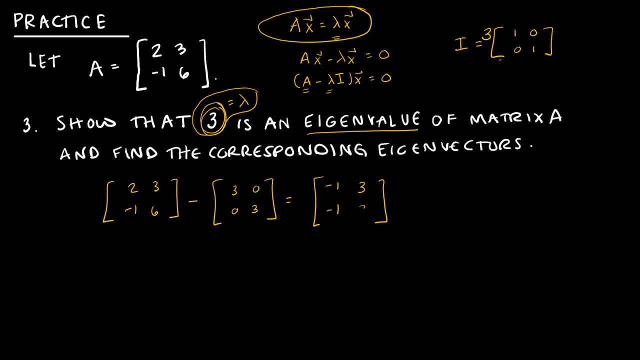 Negative. 1 minus 0 is negative, 1.. 6 minus 3 is 3.. So you might be asking: okay, great, but what am I looking for? Well, if you'll recall, our original definition said that the scalar is an eigenvalue if there is a non-trivial solution. 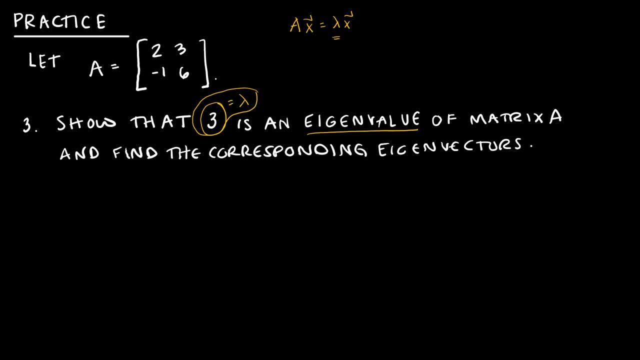 practice one, but typically you won't know that and you would have to show that it was true. You might be asking: how do we do that? Well, I'm glad you asked. We're still using this equation and we're going to say: well, if that's true, then ax minus lambda x must be equal to zero. 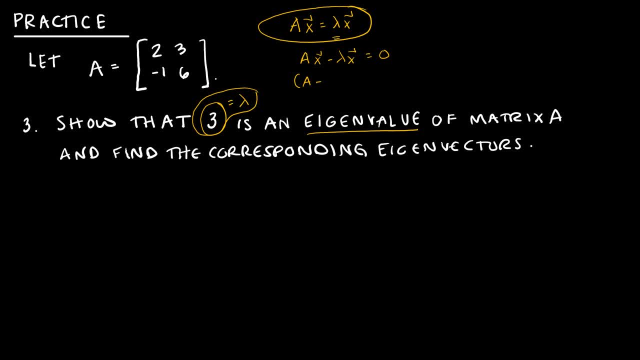 and then I could say: well, a minus lambda x is equal to zero. but can I really take a, which is a matrix, and subtract lambda, which is a scalar? No, I can't. So what am I going to do? I'm going to take lambda times the identity matrix. So for, obviously, a two by two. my identity matrix is one. 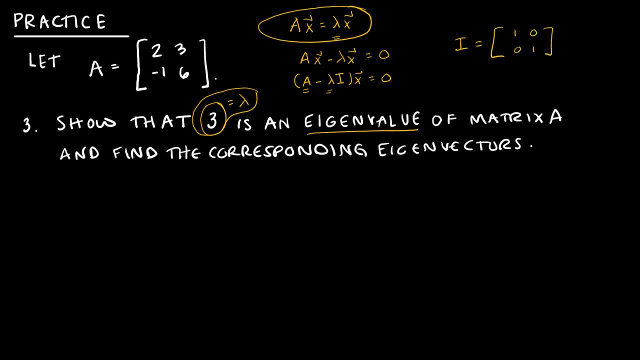 zero, zero one. So here's how this is going to work. I'm going to take a, which is two three negative one, six, and I'm going to subtract lambda, which is three times the identity matrix. So I'm going to take three times the identity matrix and get three, zero zero three, and I'm going to subtract this. 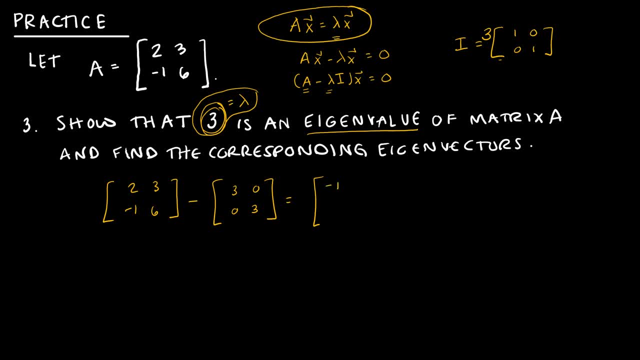 So two minus three negative one. three minus zero is three negative. one minus zero is negative one. six minus Three is three. So you might be asking: okay, great, but what am I looking for? Well, if you'll recall, our original definition said that the scalar is an eigenvalue if there is a non-trivial solution. So let's. 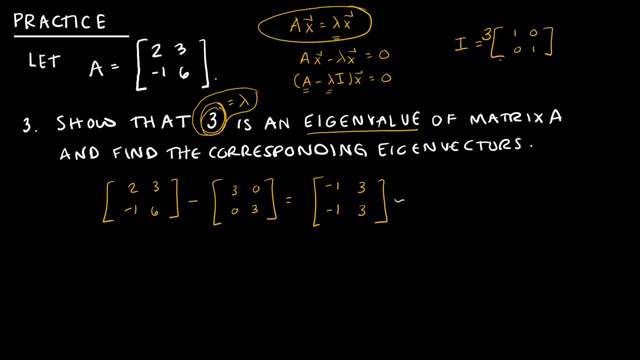 remember that if I end up, like I do here, with a free variable, because what's going to happen? I'm going to reduce this by making this positive. I'm going to reduce this by making this positive One, negative three, and then I can obviously get zero. zero here, which tells me that x one is a pivot. 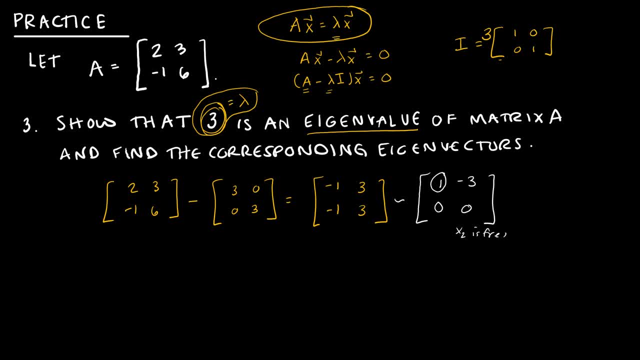 and x two is free. Why is this important? Because if I ended up with the identity matrix, then that would tell me that I had only the trivial solution. And if I have only the trivial solution, Then it's not an eigenvalue and that's not what I have. What I have is a free variable. 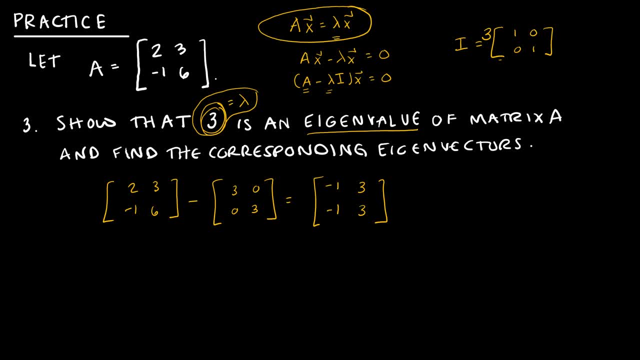 So let's remember that if I end up, like I do here, with a free variable, because what's going to happen? I'm going to reduce this by making this positive 1, negative 3. And then I can obviously get 0, 0 here, which tells me that x1 is a pivot. 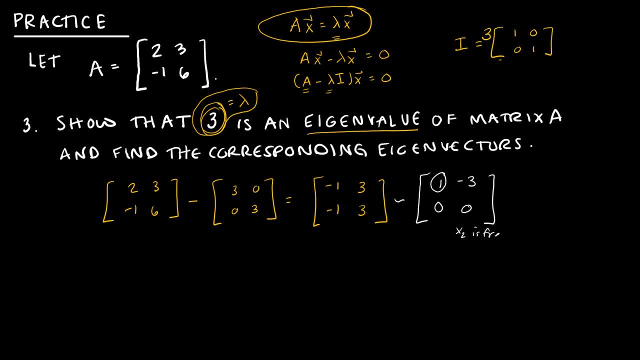 And x2 is free. Why is this important? Because if I ended up with the identity matrix, then that would tell me that I had only the trivial solution. And if I have only the trivial solution, then it's not an eigenvalue And that's not what I have. 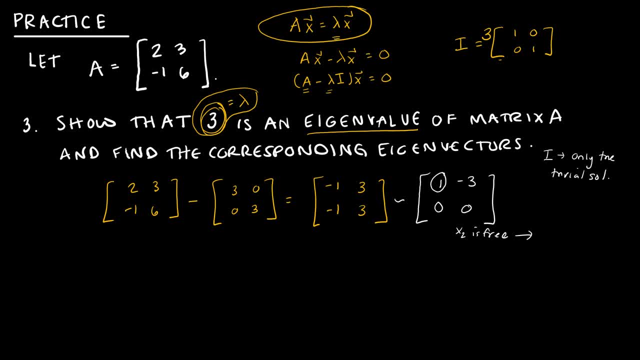 What I have is a free variable, And when you end up with a free variable, then obviously we have a non-trivial solution and therefore it's an eigenvalue. So what I've done so far is answer the first part of this question, that says, show that 3 is an eigenvalue. And by doing these, 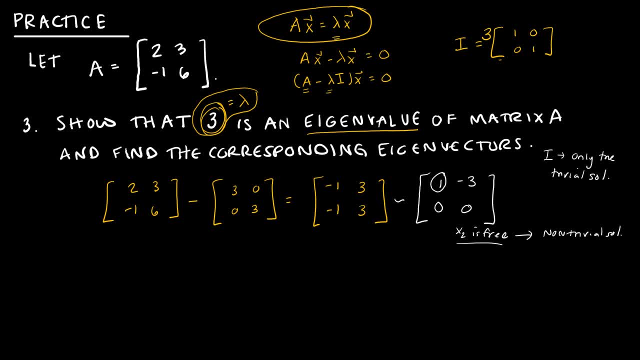 calculations and finding that I have a free variable, I have shown that in fact 3 is an eigenvalue. The next part of this question says: find the corresponding eigenvectors. Not a lot more work here and in fact work that we're quite used to. This row says, and again: 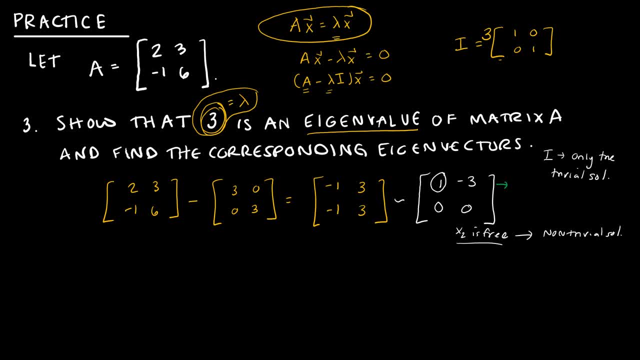 I didn't augment the matrix with 0, and if you look in your textbook, it does in fact show the zero zero column vector for the augmented matrix. But what this is telling me is as x1-x-3.. 3x2 is equal to 0.. So again, we're very used to this. We know that I can describe my solutions. 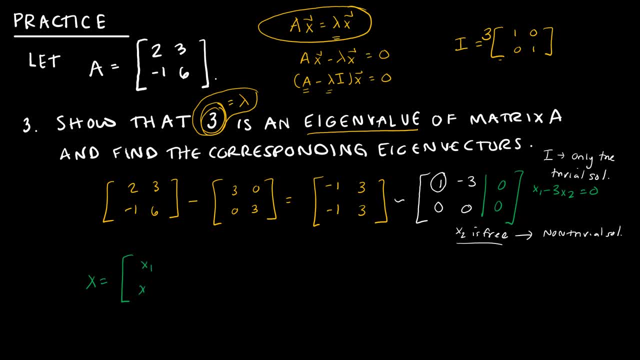 by writing x1 and x2, and that would give me x1 is actually, by moving that to the opposite side, 3x2, and x2 is x2, and I can factor out my x2, and I would get 3, 1.. 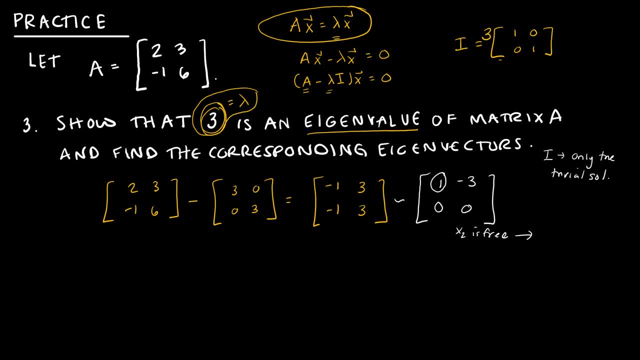 and when you end up with a free variable, then obviously we have a non-trivial solution and therefore it's an eigenvalue. So what I've done so far is answer the first part of this question, that says: show that three is an eigenvalue, and by doing these calculations and finding that, 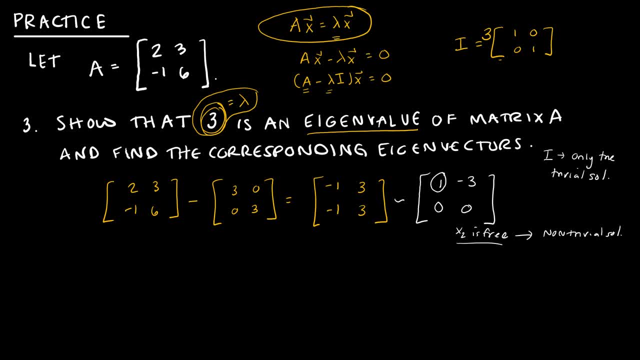 I have a free variable. I have shown that, in fact, this is something that is still valid for us, So that's something that you'll want to take a look at in your problems group. You know it's. it's important to- And, in fact, three is an eigenvalue. 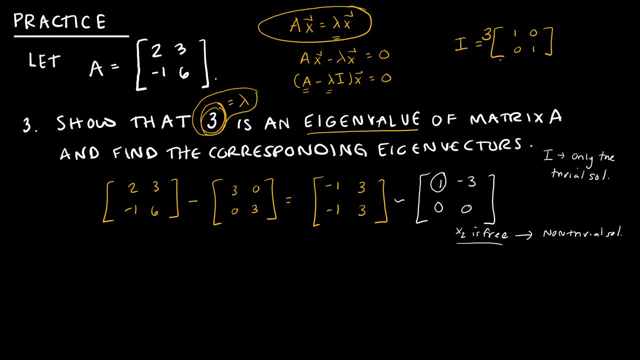 The next part of this question says: find the corresponding eigenvectors. So not a lot more work here, And in fact work that we're quite used to. This row says: and again, I didn't augment the matrix with zero. 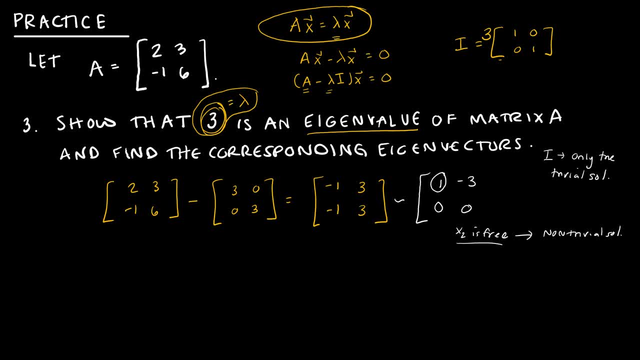 And if you look in your textbook, it does in fact show the zero column vector for the augmented matrix, But what this is telling me is as x1 minus 3x2 is equal to zero. So again, we're very used to this. 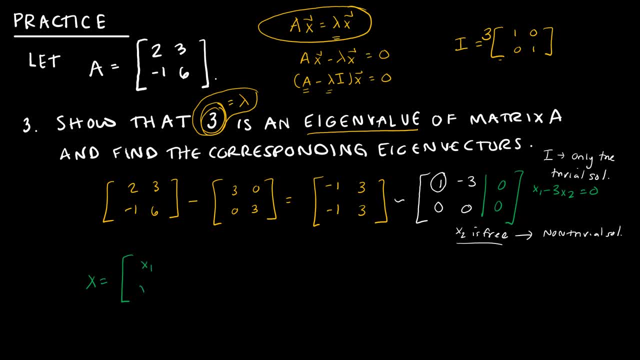 We know that I can describe my solutions by writing x1 and x2.. And that would give me x1 is actually, by moving that to the opposite side, 3x2.. And x2 is x2.. And I can factor out my x2.. 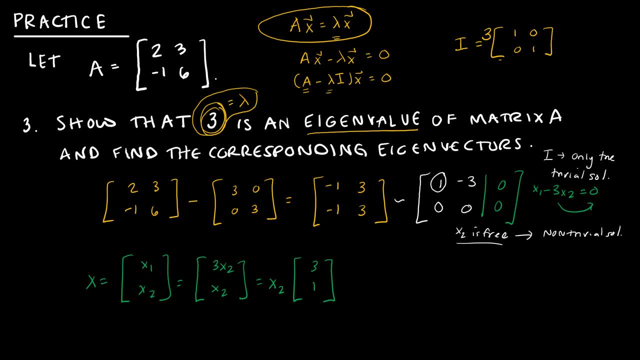 And I would get 3, 1.. So here's what I have. This is an eigenvector And this is for, specifically, the eigenvalue of 3.. The question is, how do I get the eigenvalue of 3?? 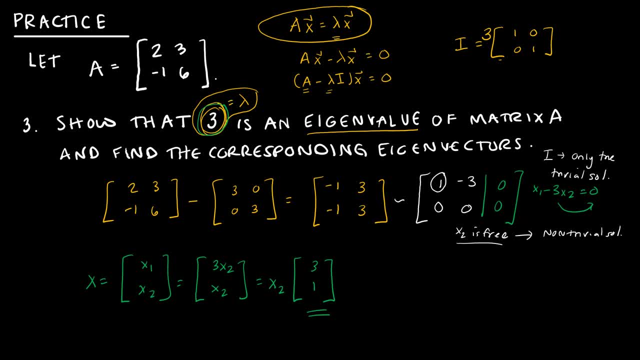 So the question says: find the corresponding eigenvectors. So the corresponding eigenvectors are all vectors in this form. So I wouldn't find, I wouldn't list all of the eigenvectors. Well, because I can't, I can only say that they're all in this form. 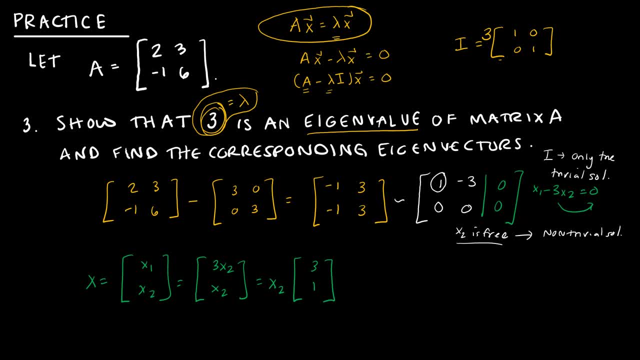 So here's what I have: This is an eigenvector and this is for, specifically, the eigenvalue of 3.. The question says: find the corresponding eigenvectors. So the corresponding eigenvectors are all vectors in this form. So I wouldn't find, I wouldn't list all of the eigenvectors. 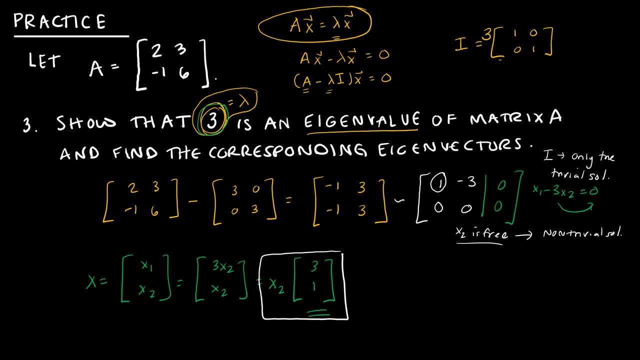 because I can't. I can only say that they're all in this form, But I want you to think about what this looks like. First of all, 3, 1 is right here And x2 is obviously a scalar, so they're saying any value I plug in for x2,. 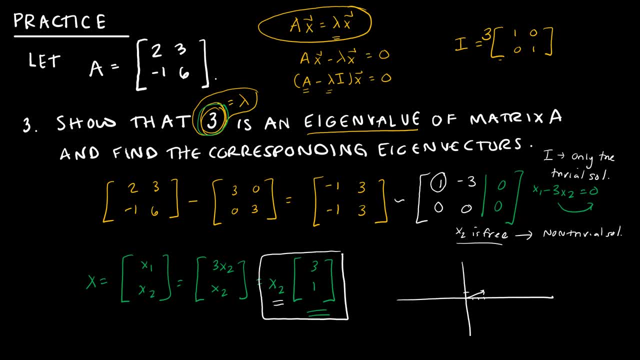 multiply that by 3, 1,, and then I would end up with some other eigenvectors. So what if I plugged in 2 for x2? Well, that would give me 6, 2.. Where is 6, 2? Well, it's over here. Notice it's on the same line. 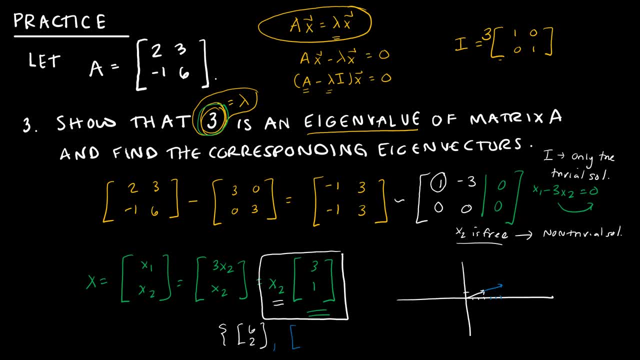 What if I plugged in negative 1?? Well, that would be negative 3, negative 1.. Where is negative 3, negative 1?? Here Why it's on the same line, And I could continue that for any values of x2, and what's going to. 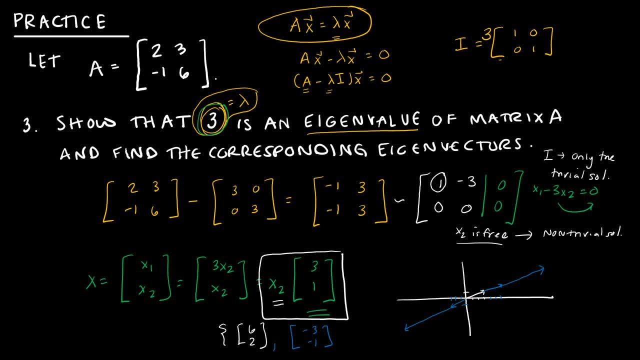 happen. I'm going to end up with values all along that line, This line, and notice that it goes through 0, 0, which is important- is called the eigenspace And again it's the null space and the subspace of Rn. So this is just a subspace and it's all the values along this line going. 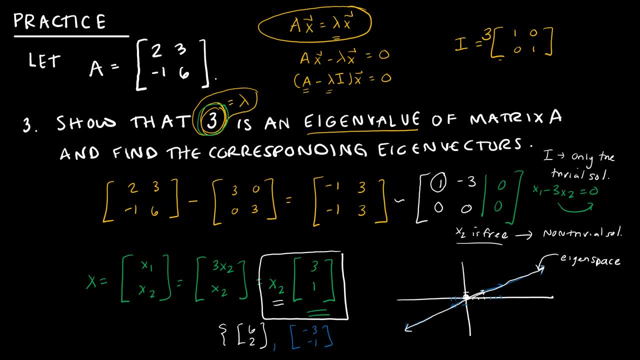 through that point: 0, 0, or 0, 0,, 0, 0, however many 0s you need. This obviously is two-dimensional. I do also want to point out that when we did questions like this before, we might be asked. 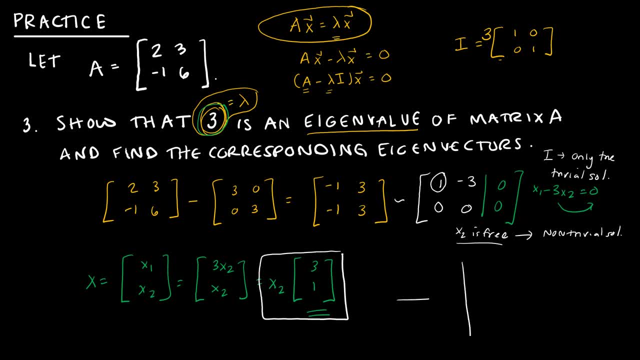 But I want you to think about what this looks like. First of all, 3, 1 is right here And x2 is obviously a scalar. So they're saying any value I plug in for x2, multiply that by 3, 1.. 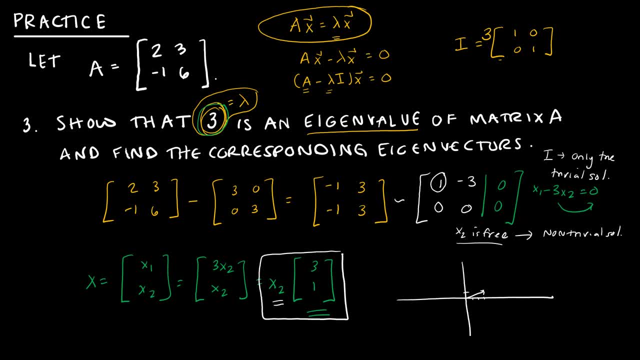 And then I would end up with some other eigenvector. So what if I plugged in 2 for x2? Well, that would give me 6, 2.. Where is 6, 2? Well, it's over here. 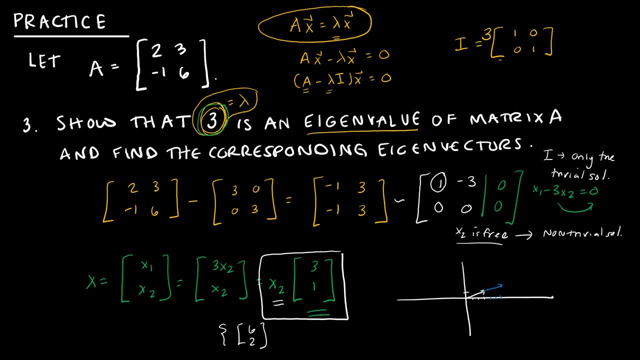 Notice it's on the same line. What if I plugged in negative 1?? Well, that would be negative 3, negative 1.. Where is negative 3, negative 1? Why, it's on the same line. And I could continue that for any values of x2.. 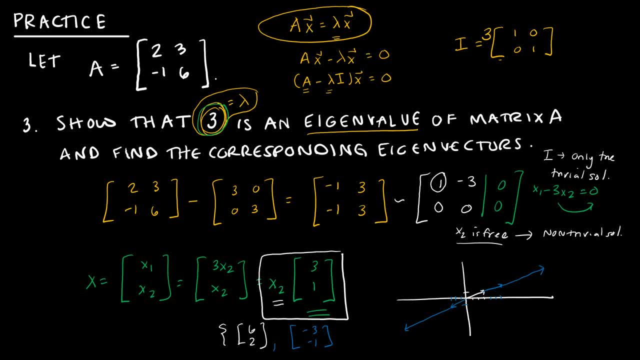 And what's going to happen. I'm going to end up with values all along that line. This line- and notice that it goes through 0, 0, which is important- is called the eigenspace And again it's the null space and the subspace of Rn. 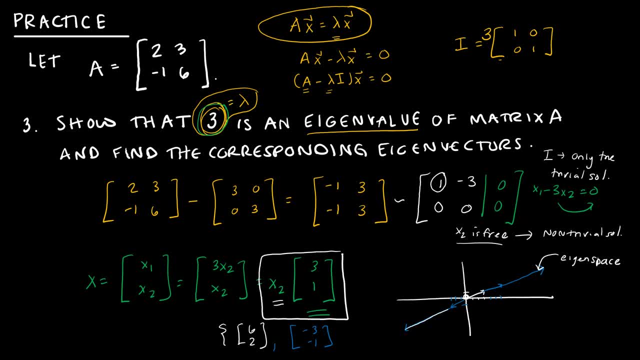 So this is just a subspace And it's all the values along this line going through that point: 0, 0.. Or 0, 0,, 0, 0,, however many 0s you need. This obviously is two-dimensional. 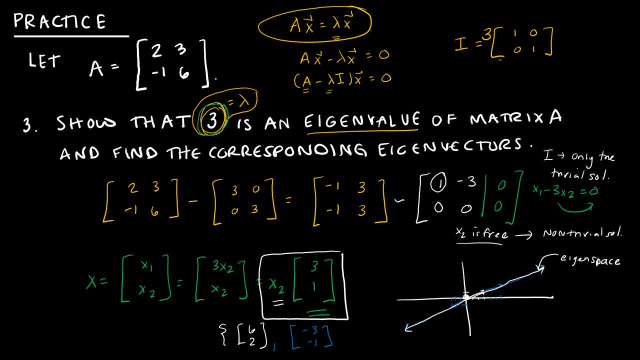 I do also want to point out that when we did questions like this before, we might be asked to find a basis. Well, that's really what I have done already. This is obviously a 2x2 matrix, And when I'm finding the basis- which I have already done the work for- 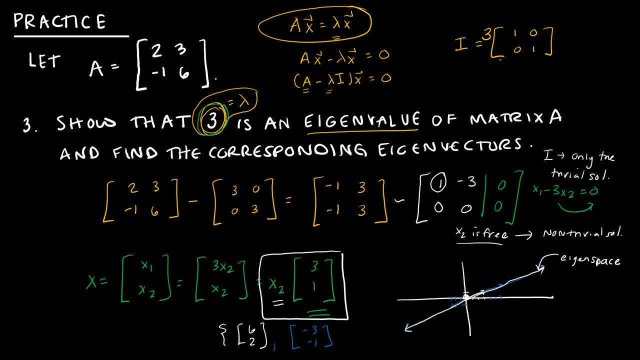 to find a basis. Well, that's really all. we need to find a basis. We're going to need to find a basis. Well, that's really all we need to find a basis. We're going to need to find a basis. Well, that's really. 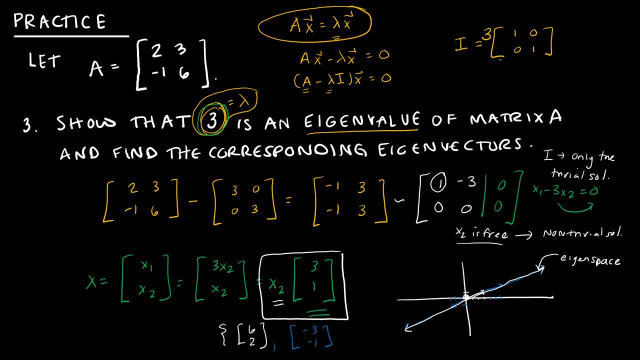 all. we need to find a basis. We're going to need to find a basis. We're going to need to find a basis. What I have done already, This is obviously a two-by-two matrix, and when I'm finding the basis, 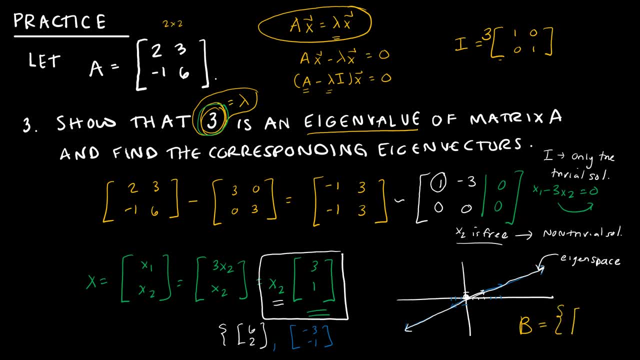 which I have already done the work for it's just going to be that 3, 1.. And, if you'll notice, I have one vector for a two-by-two and it makes perfect sense for that, because I have a two-by-two matrix and I have a two-by-two matrix and I have a two-by-two matrix. 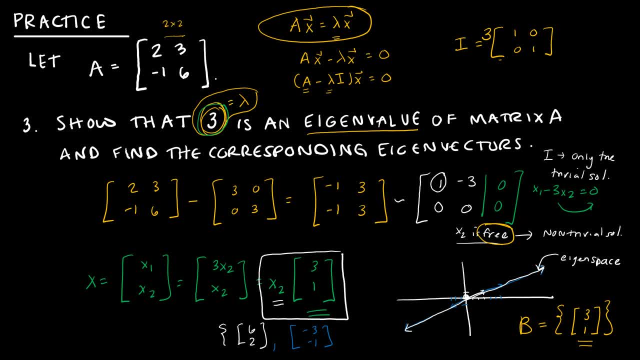 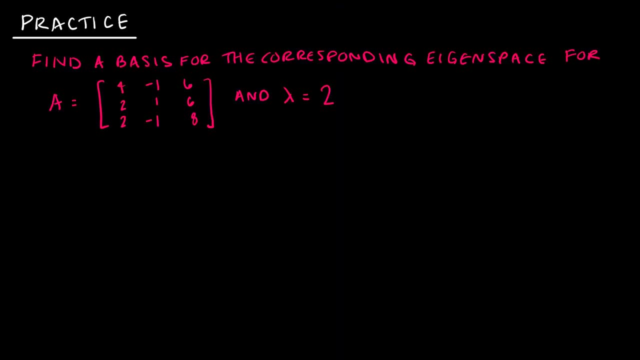 and I have a free variable. So it wouldn't make sense to have two vectors in a two-by-two matrix, unless you know, I was having only the trivial solution, which would mean it wouldn't work anyway. So you should always have one fewer. Let's try another question where we are asked. 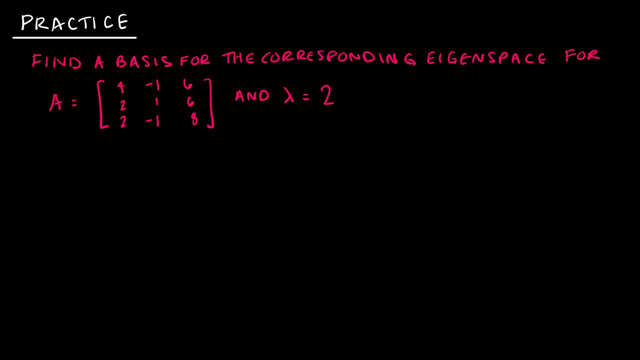 to find the basis. And again, this one is a three-by-three matrix and we are given again the eigenvalue of two and we are asked to find the basis for the corresponding eigenspace. So again, all I'm going to do is use that same formula. 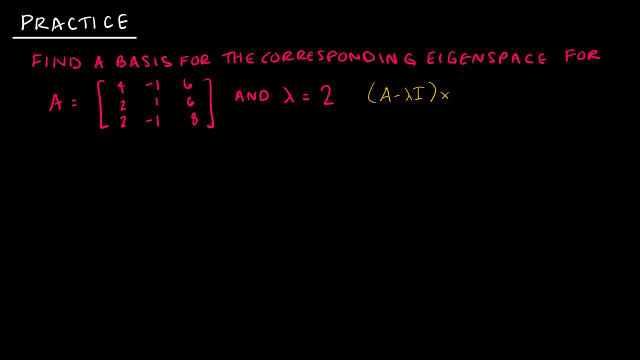 a minus lambda i x equal to 0. So in this case that means 4, negative, 1, 6, 2, 1, 6, 2, negative, 1, 8, subtracting 2 times the identity matrix, so 2, 0, 0,. 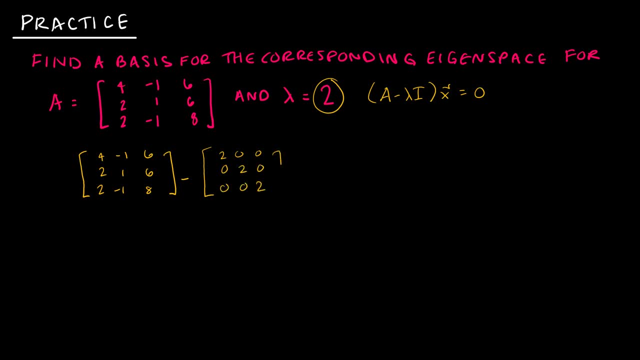 0, 2, 0, 0, 0, 2.. Subtracting gives me 2, negative: 1, 6, 2, negative 1, 6, 2, negative 1, 6.. 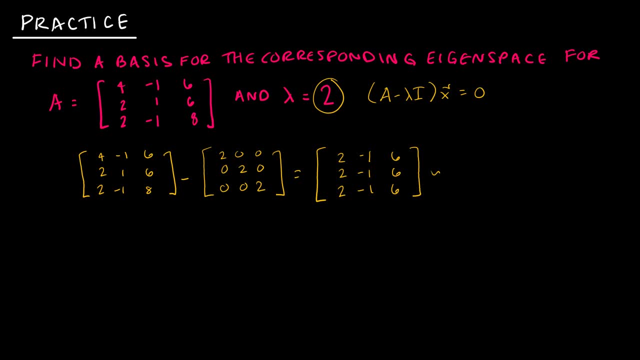 Doing row operations. obviously I end up at 2, negative, 1, 6, 0, 0, 0, 0, 0, 0.. And I could continue further to get 1, negative, 1, half, 3, 0, 0, 0, 0, 0, 0.. 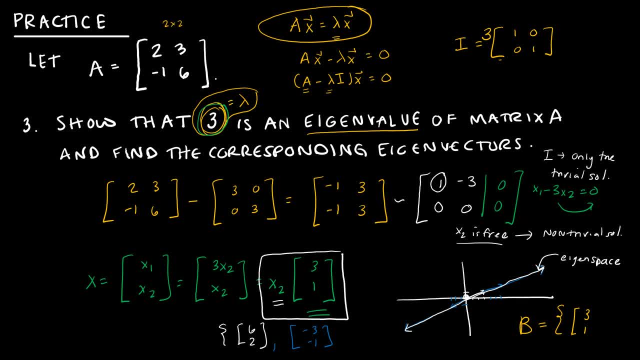 it's just going to be that 3, 1.. And, if you'll notice, I have one vector for a 2x2.. And it makes perfect sense for that because I have a free variable. So it wouldn't make sense to have two vectors in a 2x2 matrix. 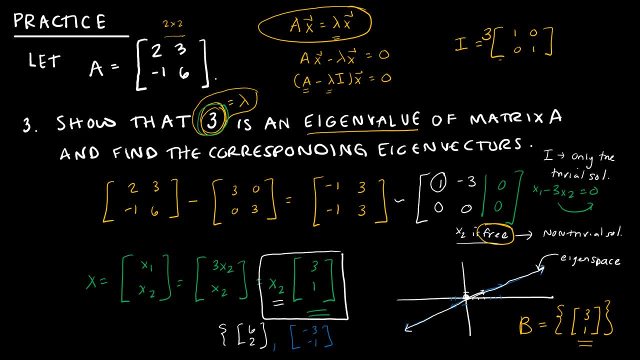 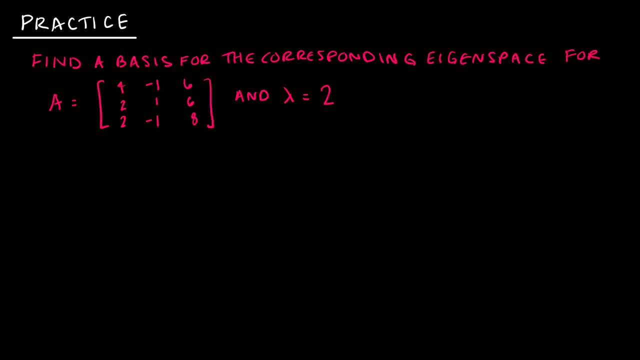 unless I was having only the trivial solution, which would mean it wouldn't work. So you should always have one fewer. Let's try another question where we are asked to find the basis, And again this one is a 3x3 matrix. 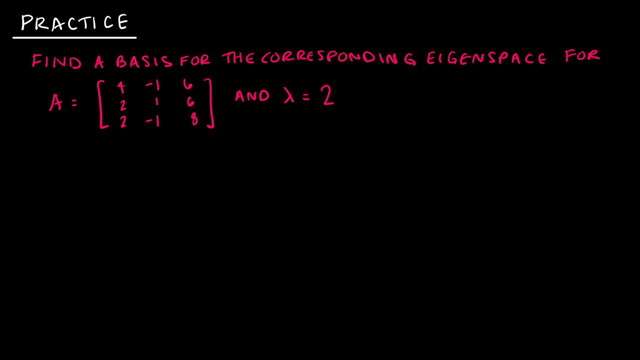 And we are given again the eigenvalue of 2. And we are asked to find the basis for the corresponding eigenspace. So again, all I'm going to do is use that same formula: a minus lambda i, x equal to 0.. 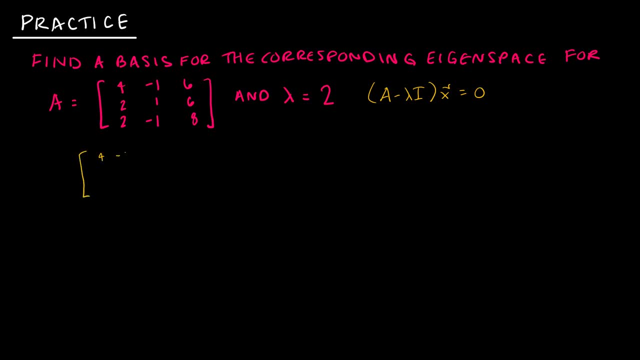 So in this case that means 4, negative, 1, 6, 2, 1, 6, 2, negative 1, 8, subtracting 2 times the identity matrix, So 2, 0, 0, 0, 2, 0, 0, 0, 2.. 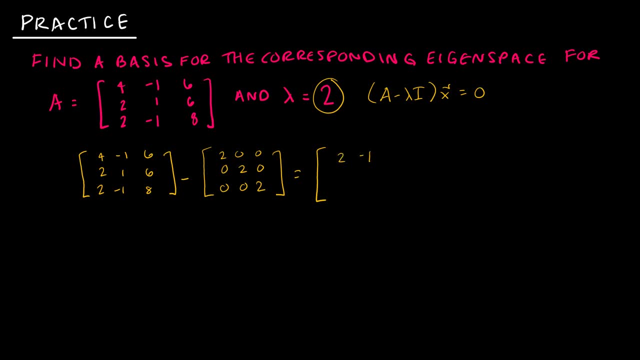 Subtracting gives me 2, negative 1, 6, 2, negative 1, 6, 2, negative 1, 6.. Doing row operations, obviously I end up at 2, negative 1, 6, 0, 0, 0, 0, 0, 0.. 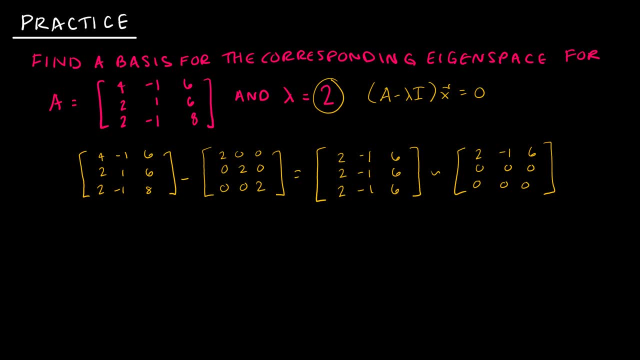 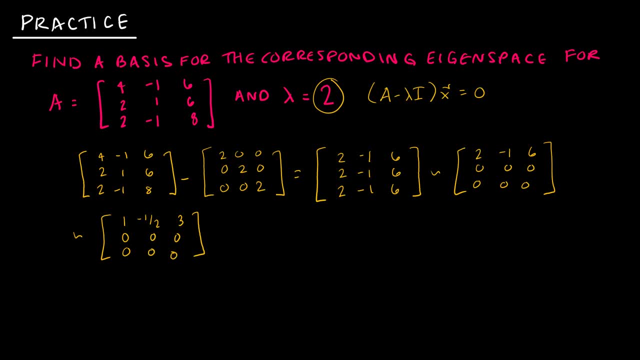 0, 0, 0, which means, of course, that I can write this: as we have X 1, X 2, X, 3, X, we have X 1, and then my free variables are, of course, X 2 and X 3, which means I can write X 1. I'm just going to go straight to having X 2 and X 3 on the outside. 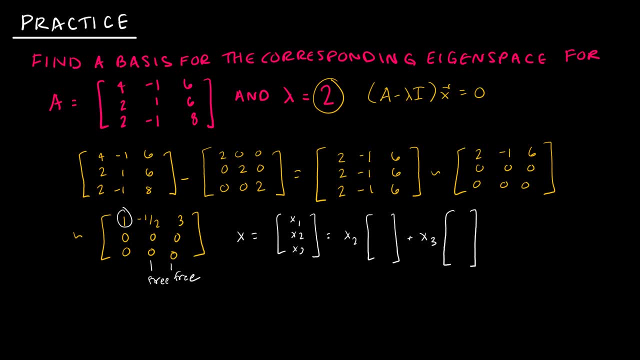 so X 1 can be written as 1, half X 2 minus 3 X 3, and then of course X 2 is X 2, and then 0 X 3 and X 3 is X 3. so again the question says: 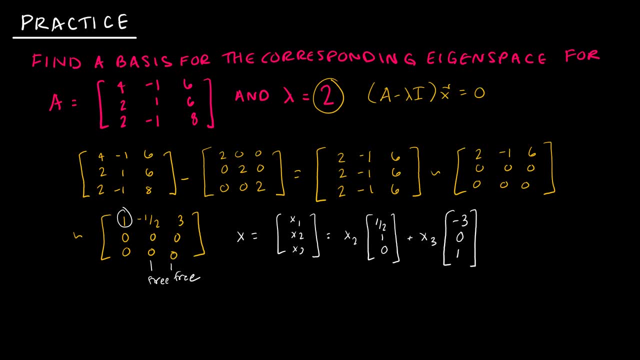 find the basis. So what I have done is write it in its general form, which means my basis is those I keep forgetting to put those brackets is: one half one zero and negative three zero one And again, just as we talked about last time, this is a three by three matrix. 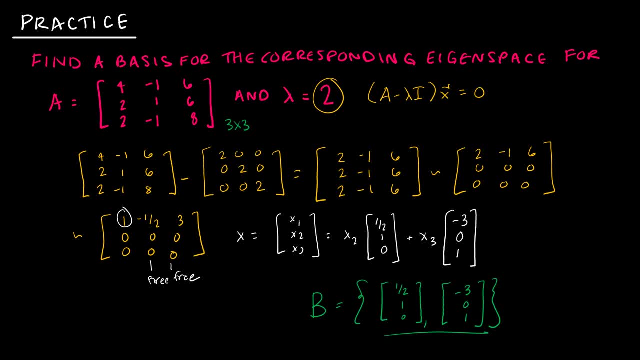 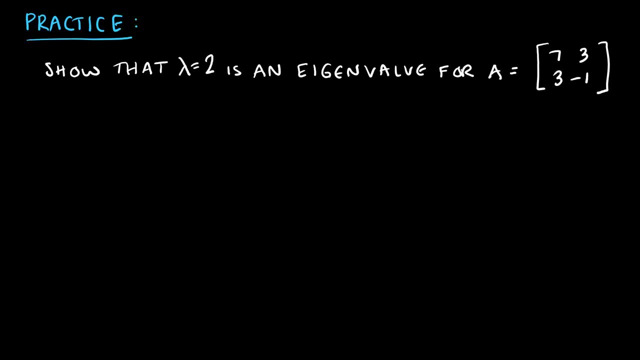 but notice, I'm only going to have two vectors in my basis. I do have this one last practice for you to try on your own, but before you do it, I just want to point out that section 5.1, I've really broken it into two parts- This video, that 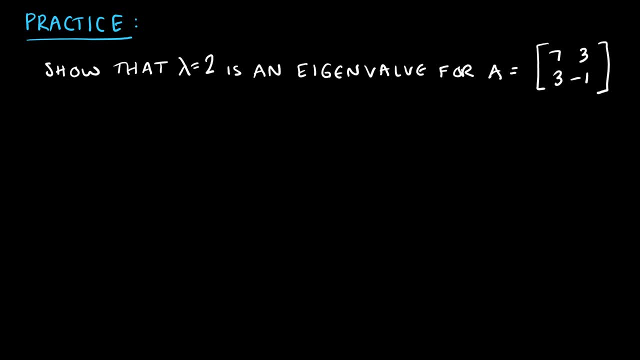 you're watching now is the very practical. here's how you actually do it video. The next video is the very practical. here's how you actually do it video. The next video is the very practical, more theoretical video. So we're going to be looking at a couple of theorems dealing with 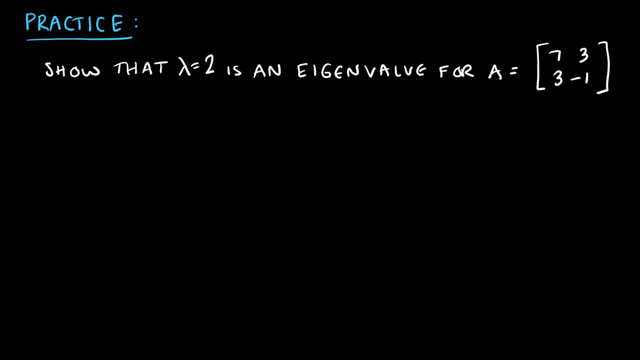 eigenvectors and eigenvalues. So back to this question. This should be very similar to the last two questions that we did. I want you to show that lambda equals two is an eigenvalue, or show that it is not. Once you are done, press play to see how you did. 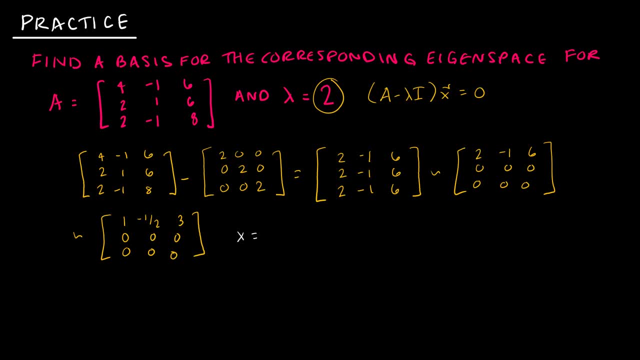 Which means, of course, that I can write this: as we have x1, x2, x3, x, we have x1.. My free variables are, of course, x2 and x3.. Which means I can write x1. 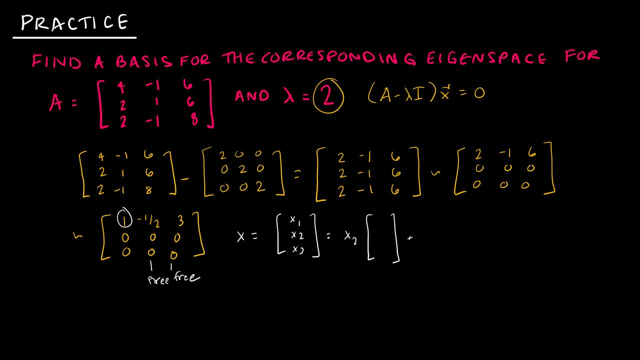 I'm just going to go straight to having x2 and x3 on the outside. So x1 can be written as 1, half x2 minus 3x3. And then of course x2 is x2. and then 0x3 and x3 is x3. So again the question says: find the basis. So what I have done, 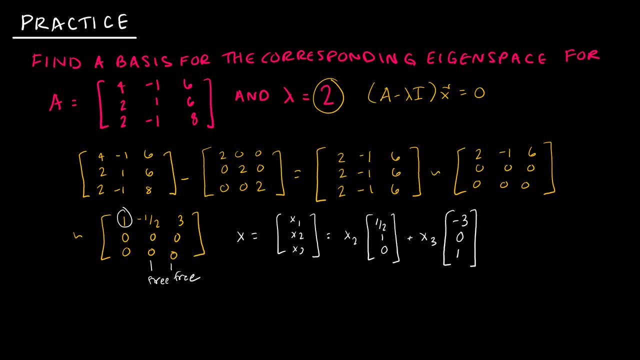 is write it in its general form, which means my basis is those. I keep forgetting to put those brackets is 1, half 1, 0 and negative 3 0, 1.. And again, just as we talked about last time, 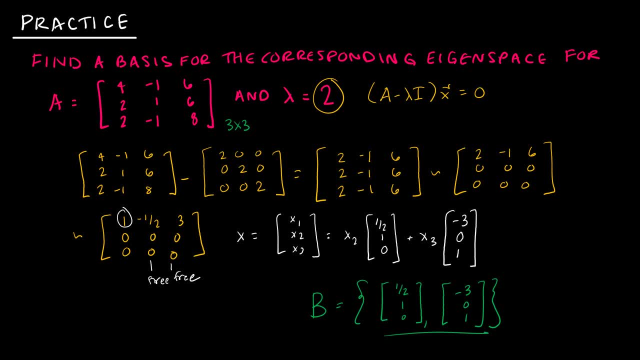 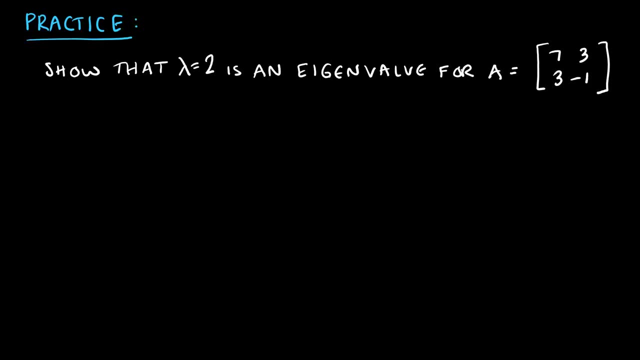 this is a 3x3 matrix, but notice, I'm only going to have two vectors in my basis. I do have this one last practice for you to try on your own, but before you do it, I just want to point out that 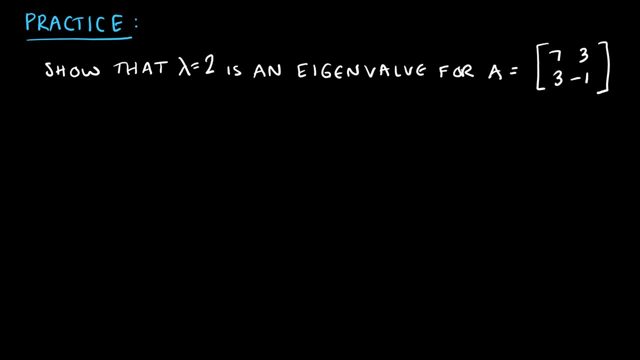 so Section 5.1, I've really broken it into two parts. This video that you're watching now is the very practical. here's how you actually do it video. The next video is the more theoretical video. so we're going to be looking at a couple of theorems dealing with eigenvectors and eigenvalues. 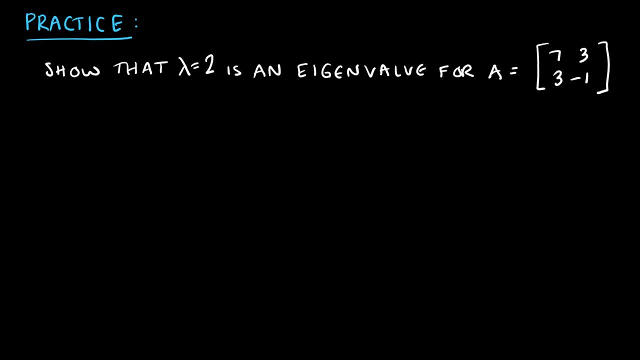 So back to this question. This should be very similar to the last two questions that we did. I want you to show that lambda equals 2 is an eigenvalue, or show that it is not. Once you are done, press play to see how you did. 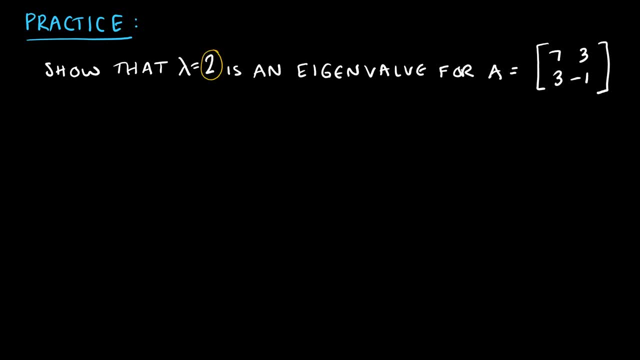 So no surprises here. I'm using an eigenvalue of 2, and I'm going to take a which is 7, 3, 3, negative 1. I'm going to subtract 2 times the identity, So again I've got a minus lambda. 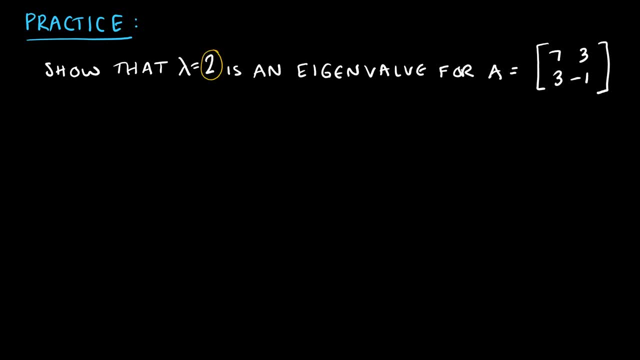 So no surprises: here I'm using an eigenvector, excuse me, an eigenvalue, and I'm going to take a which is 7, 3, 3, negative 1.. I'm going to subtract 2 times the identity, So again I've got a minus lambda i x equal to 0.. So I'm taking 2, 0,, 0,, 2.. 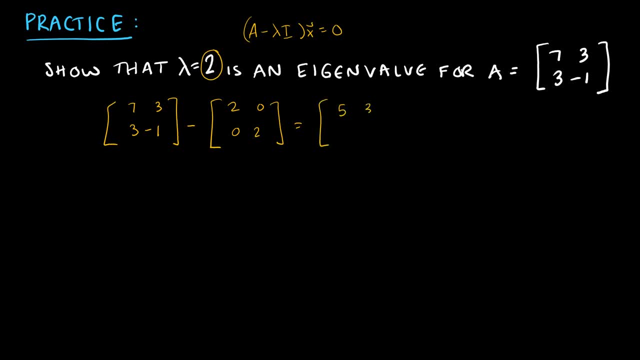 7 minus 2 is 5,, 3 minus 0 is 3,, 3 minus 0 is 3, and negative 1 minus 2 is negative 3, and I should be able to stop right here, because it's very clear to me that I can start doing. 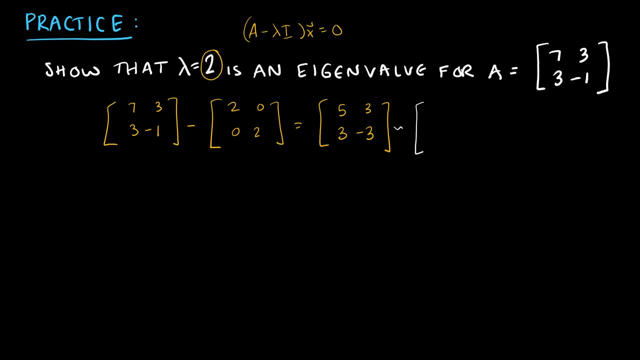 some row operations and I'm going to go ahead and reduce this, But hopefully at this very first point, before I ever do row operations. you can see that I'm not going to end up with a free variable. But in case you can't, that's okay, Let's add rows 1 and 2 together. That's going to give me 8 here. 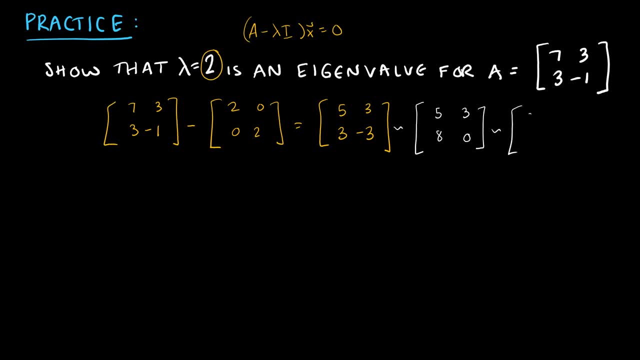 and 0 here, And I'm going to do a row swap because I want my first value to be to be 1.. So I'm going to now take 1, 8th, So I'm doing a scalar, So I have 1, 0,. 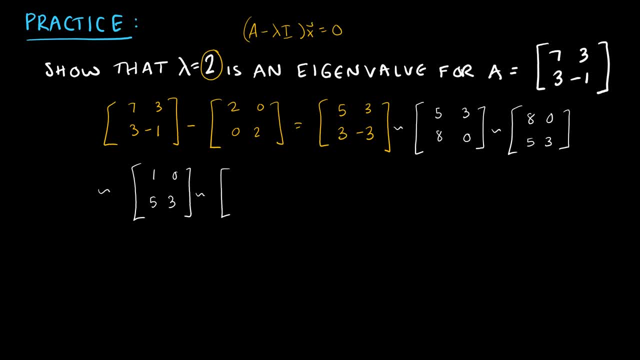 5, 3.. I can take negative 5 times row 1 and end up with 0 and negative 2.. I'm sorry, just kidding 0 and 3.. And then I can do 1, 3 of row 2 and end up with 1, 0,, 0, 1.. But again, hopefully when you got to this point. 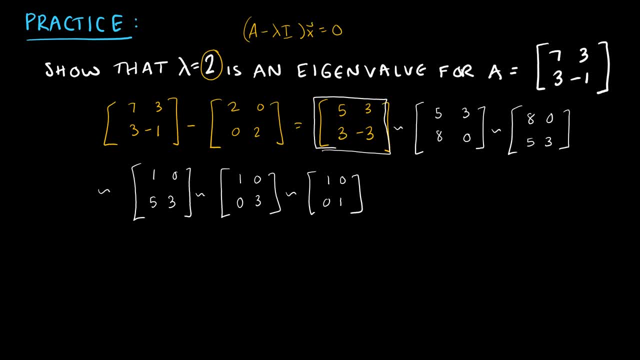 you could see what the outcome was going to be. But even if you couldn't, what I've ended up with now is the identity matrix. Now, if you'll keep in mind what we did before, I had a free variable before, and the free variable before told me that I had more than just the trivial solution. 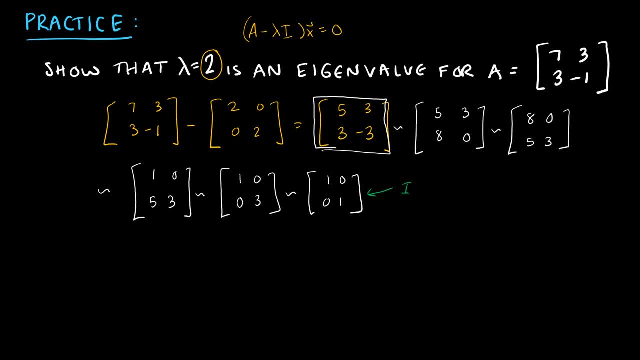 This guy is the identity matrix, Which means I have only the trivial solution. And what does only the trivial solution tell me? That lambda equals 2 is not an eigenvalue for matrix A. 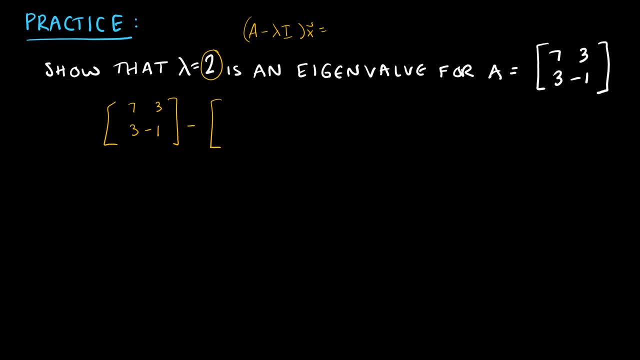 equals 2.. I x equal to 0.. So I'm taking 2, 0, 0,, 2.. 7 minus 2 is 5.. 3 minus 0 is 3.. 3 minus 0 is 3.. 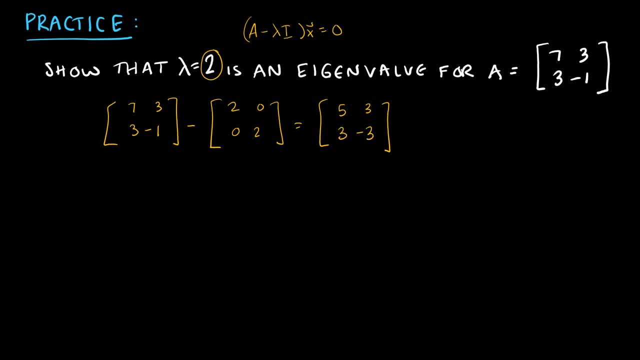 And negative 1 minus 2 is negative 3.. And I should be able to stop right here, because it's very clear to me that I can start doing some row operations And I'm going to go ahead and reduce this, But hopefully at this very first point, before I ever do row operations. you can see, 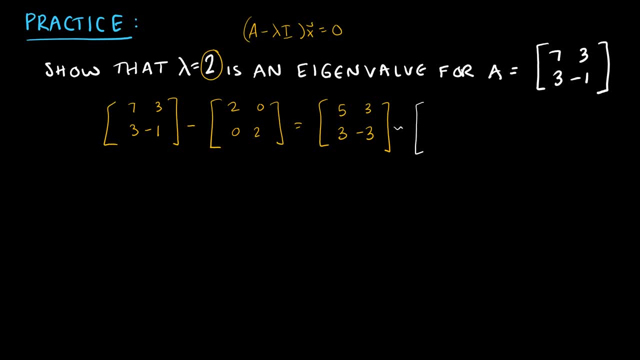 that I'm not going to end up with a free variable, But in case you can't, that's okay, Let's add rows 1 and 2 together. That's going to give me 8 here and 0 here, And I'm going to do a row swap because I want my first value to be 1.. So I'm going to now take 1. 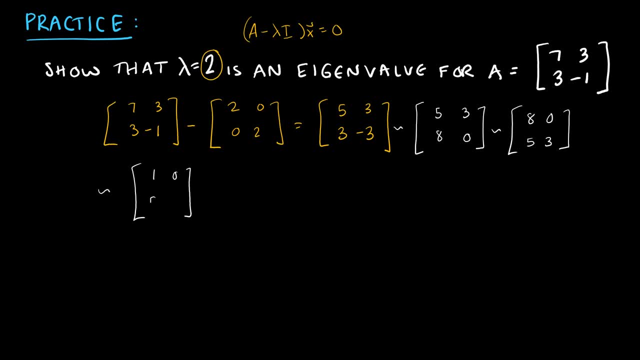 eighth. So I'm doing a scalar. So I have 1, 0,, 5,, 3.. I can take negative 5 times row 1 and end up with 0 and negative 2.. I'm sorry, Just kidding- 0 and 3. And then I can do 1 third of row 2 and end up with 1, 0, 0, 1.. 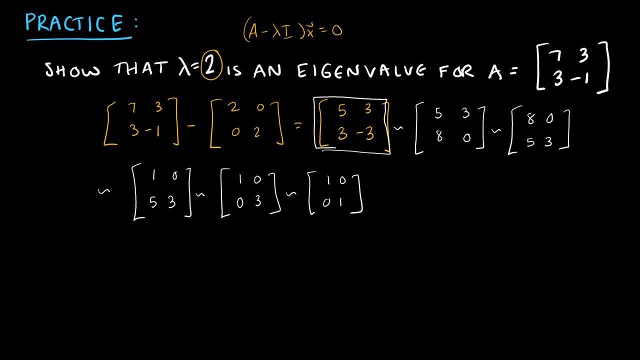 But again, hopefully, when you got to this point, you could see what the outcome was going to be. But even if you couldn't, what I've ended up with now is the identity matrix. Now, if you'll keep in mind what we did before, I had a free. 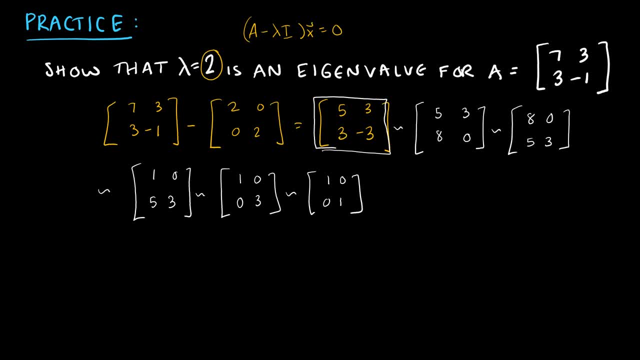 variable before and the free variable before told me that I had more than just the trivial solution. This guy is the identity matrix, which means I have only the trivial solution. And what does only the trivial solution tell me? That lambda equals 2 is not an eigenvalue for matrix A.